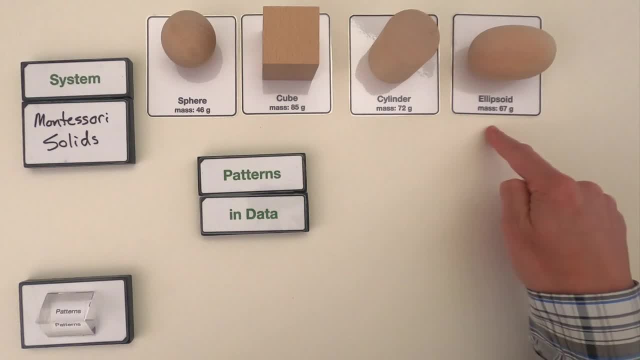 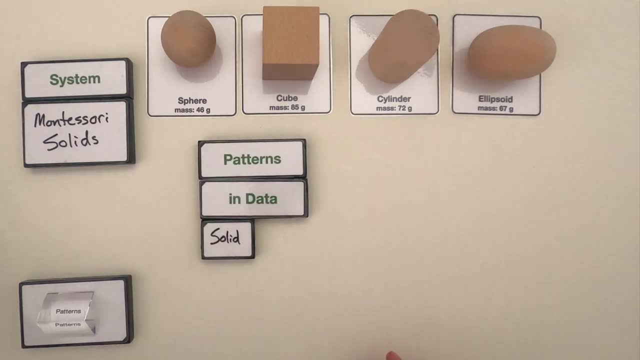 You can see that some of the data is already provided for us. You can see the mass of each of these, And so let me list some of the patterns that I see. So the big patterns that I see is the different types of solids, the mass of each solid, the 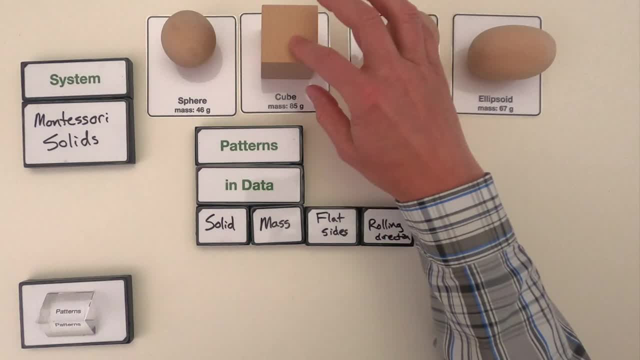 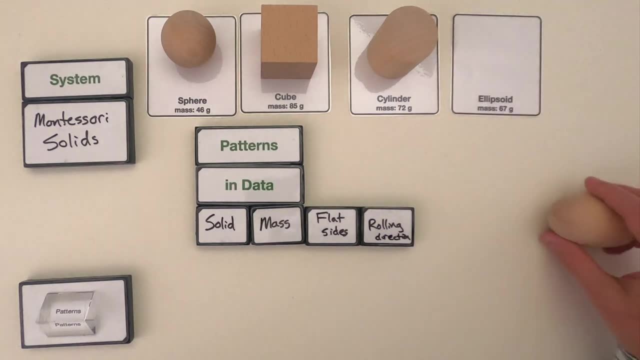 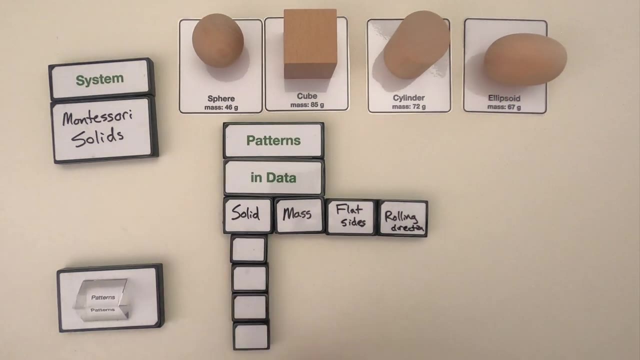 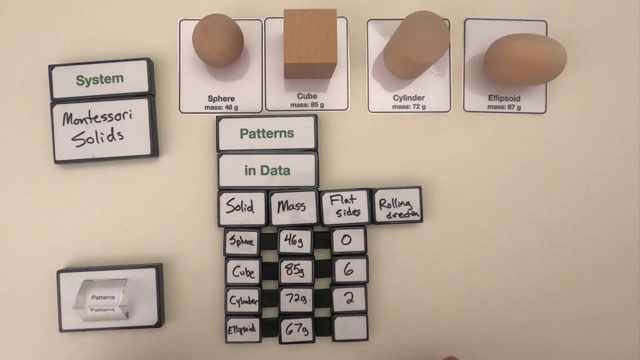 number of flat sides, and then the rolling direction. You have things like a cube that doesn't roll, a cylinder that can only roll in two directions, and then something like a sphere or an ellipsoid that can roll in many different directions, And so let me list some of those patterns down below. 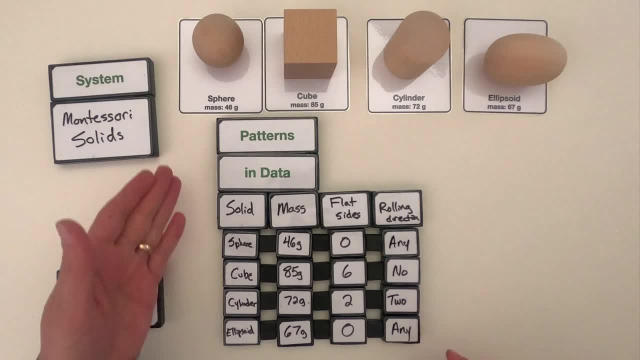 Okay, now that I've listed all the patterns in the data, what I can start to do is just analyze patterns within a data set. Okay, now that I've listed all the patterns in the data, what I can start to do is just analyze patterns within a data set. 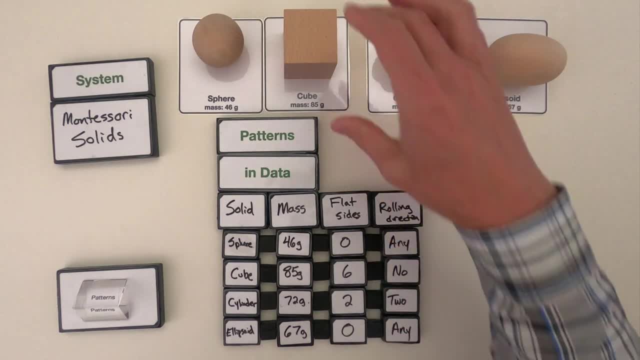 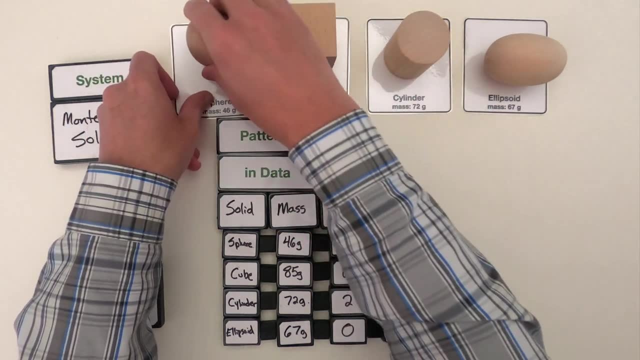 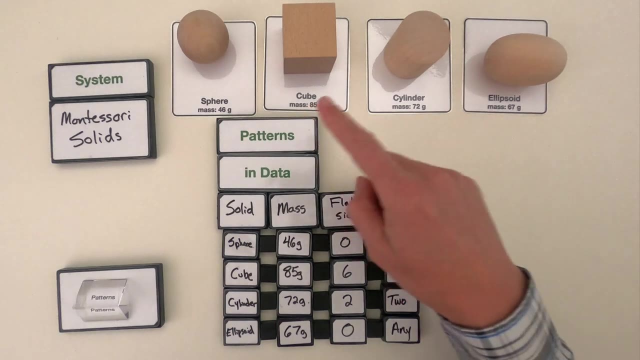 So if I'm looking at mass, what's something interesting? The cube is going to be the most massive, So this is going to be really heavy compared to something like a sphere. What are some other things that I notice is that the sphere and the ellipsoid can roll in any direction. 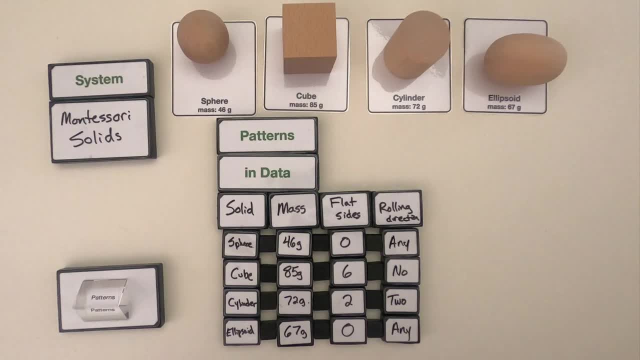 So I'm looking at patterns within each data set And then I can start comparing data sets. So how is the number of flat sides related to the rolling direction? So a pattern that I know is the rolling direction. What I notice is if you have zero flat sides, like in the sphere or the ellipsoid, you can roll in any direction. 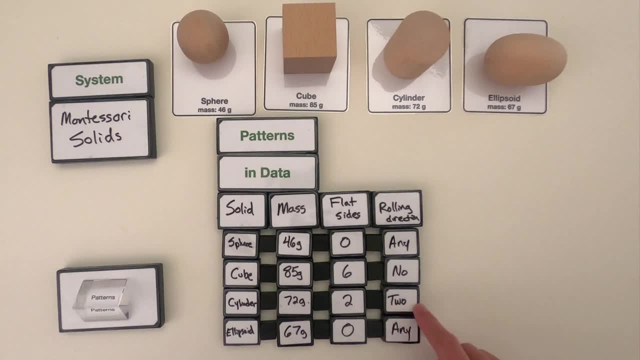 Something like a cylinder that has two flat sides can only move in two directions, And the cube that has six can't roll in any direction, And so this is just looking at patterns in data. What I'm really trying to do is dig into the data that was collected either by myself or someone else, to make sense of the system. 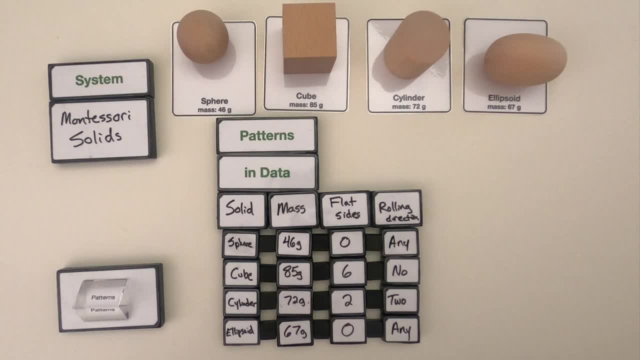 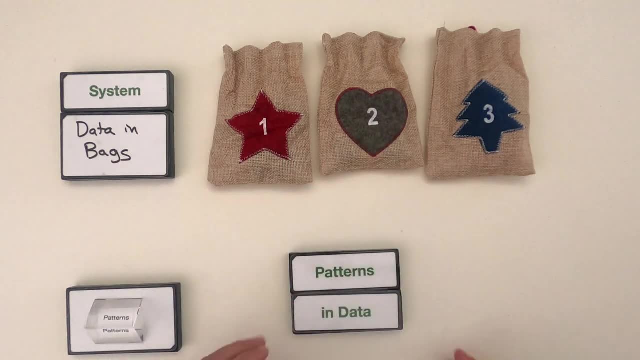 So what I'm going to do is clear this off, And then I'm going to set up another set of data, And I want you to do the same. Okay, the second system we're going to look at is some data that's been provided in these three bags. 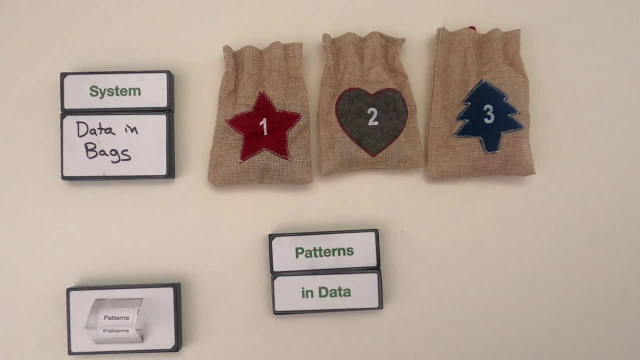 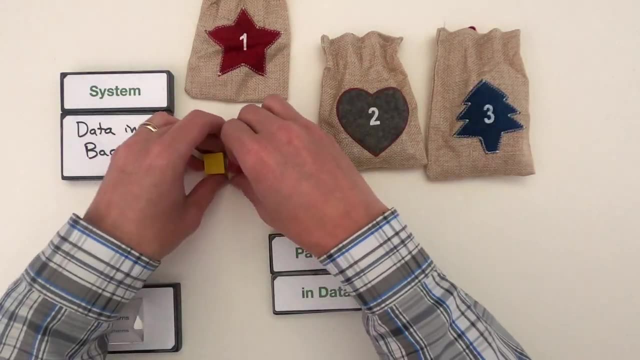 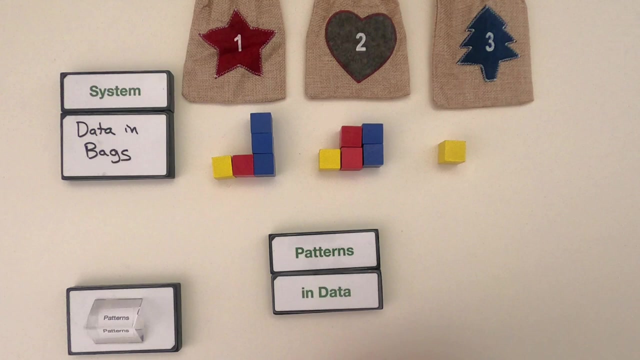 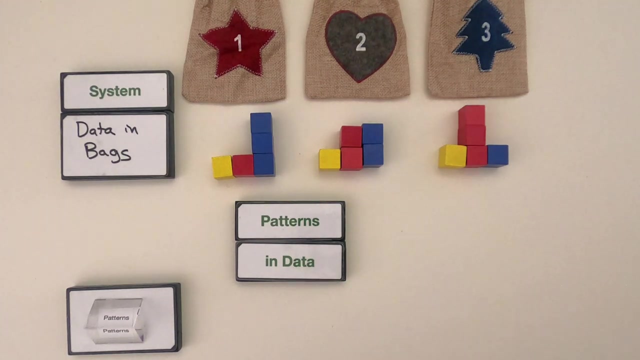 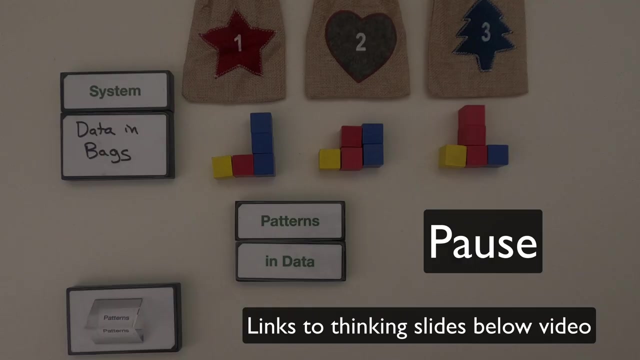 And I'm going to encourage you to pause the video and try to write down what are the patterns that you see in the data. But first let me dump out the data and then organize the data. So what I'm going to have you do is organize the patterns in the data below here, then unpause the video and then come back and we'll share our thinking. 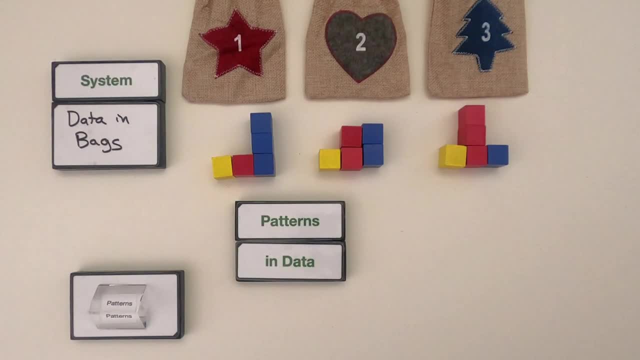 Okay, the first thing that I would do is organize this. Numbers are going to be super important when we look at this data. So let me look at all the data that we have and how I would organize the patterns. So the first pattern that I notice is that we have three different bags, and then we have different colors of each of these different cubes. 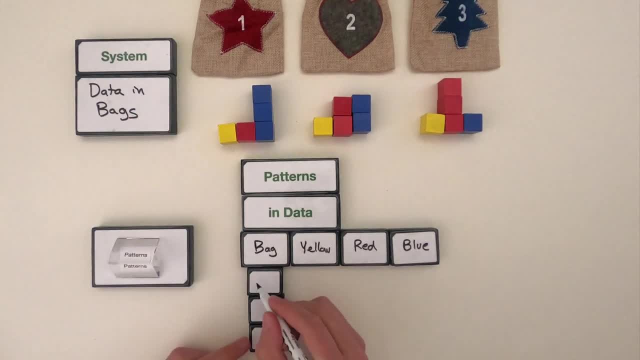 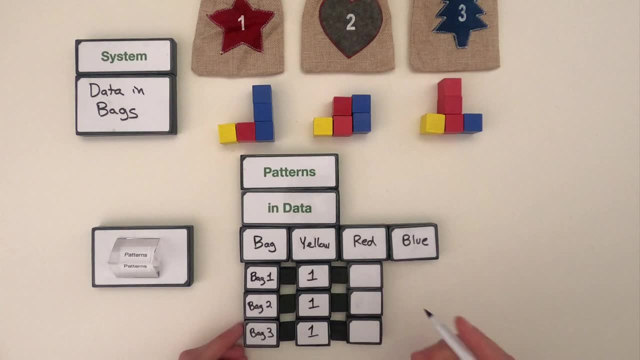 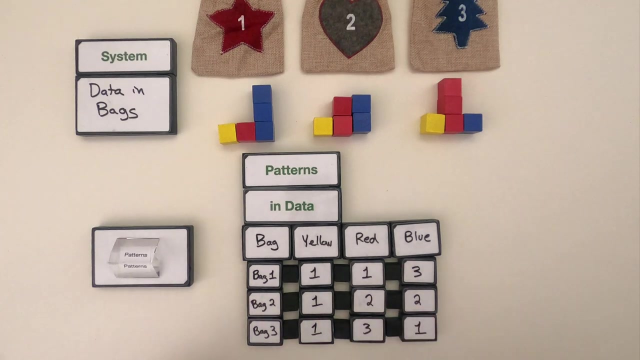 So now let me write that down below. Okay, now that I've organized the data, I start looking for patterns in the data. The best way to look for patterns in the data is to first look within the data. So I would say the bags increase from one to two to three. 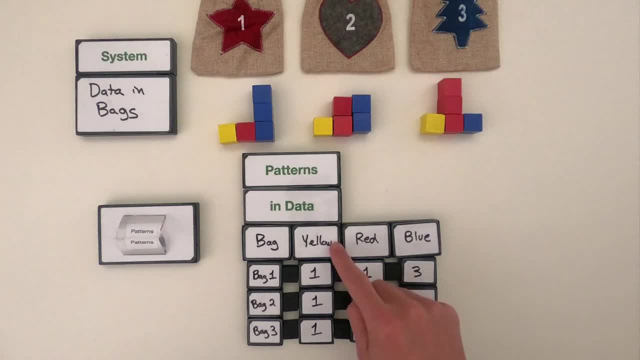 So the bag increases one, two, three. If we look at the yellow, the yellow stays the same, The red increases one each time and the blue decreases one each time. So that's the first step of looking for patterns in the data. 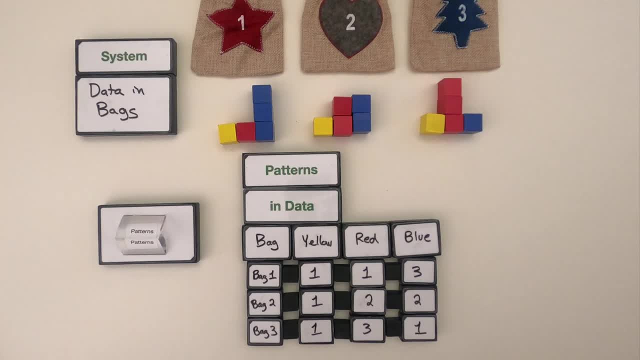 The next thing you should start doing is comparing. So what's the relationship between bag one and the red? So a way to think about that is: bag one goes to two, goes to three. Red goes from one to three. Red goes from one to two to three. 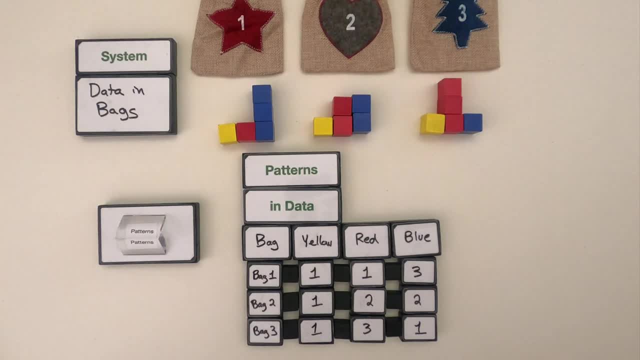 And so you could say there is a direct relationship or an increase as we look at red over the three bags. Or you could look at what's the relationship between bag one and blue. So over time, as we go from bag one to three, we see a decrease in the number of cubes in each of those. 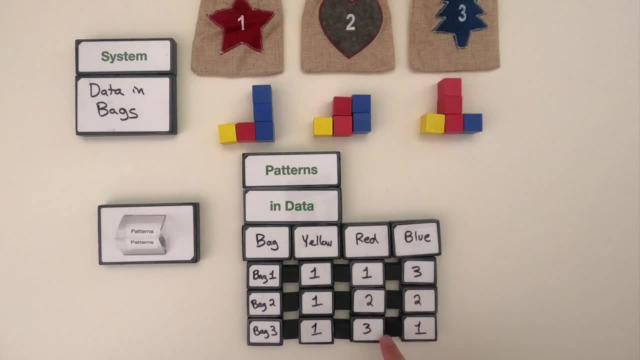 We could say there's an inverse relationship between red which goes up and blue which goes down. Or another thing we could look at is, over time, yellow stays the same. So all we're doing as we go through this is trying to figure out what story or what patterns do we see in the data?